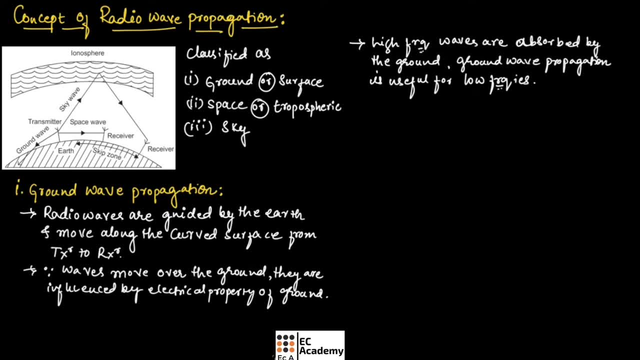 So the high frequency waves will be strongly absorbed by the ground. That is why ground wave propagation is useful for low frequencies and also the ground wave propagation is very reliable Here. the ground wave propagation will be very much reliable whatever atmospheric condition may be. 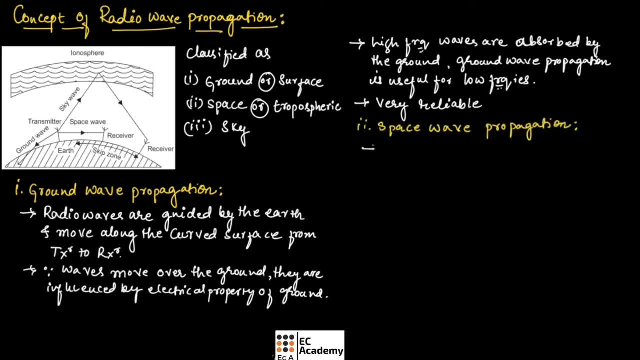 Now let us understand space wave propagation. When radio waves are transmitted by antenna, these radio waves travel in striaght line, directly reaching receiving antenna. This process is known as space wave propagation. When the radio waves are transmitted by an antenna, these radio waves travel in striaght. 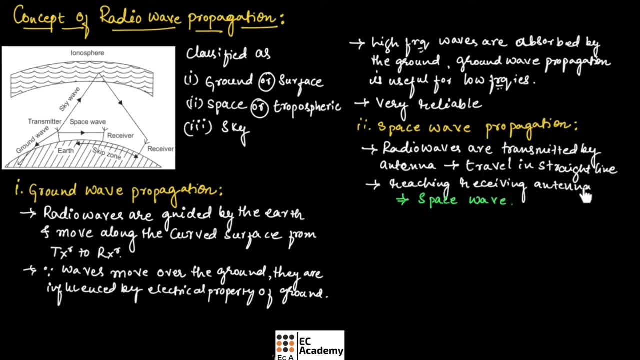 line and it will reach receiving antenna. process is known as space wave propagation. The space wave is made up of two components. First one is line of sight wave and second one is ground reflected wave. The space wave is made up of two components. 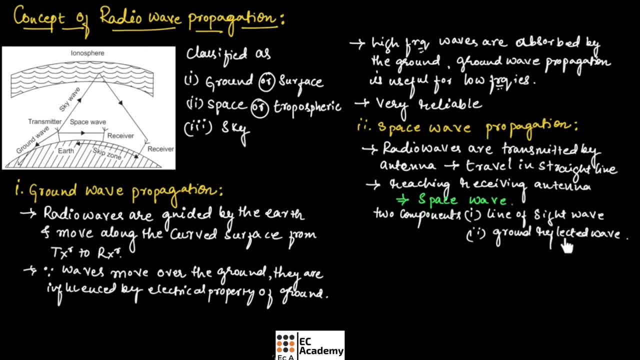 First one is line of sight wave and second one is ground reflected wave. In line of sight wave, the signal is directly transmitted from transmitter to receiver. In ground reflected wave, the signal is transmitted from transmitter and then it is reflected from the surface of the earth, and then it will reach to the receiver. 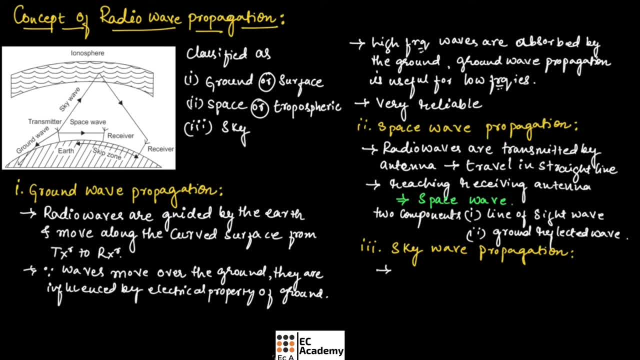 Now let us understand sky wave propagation. In sky wave propagation, radio waves are transmitted from transmitting antenna and these waves reaches The receiving antenna after reflection from the ionosphere. In sky wave propagation, the radio waves are transmitted from the transmitting antenna and these radio waves will reach the receiving antenna after reflection from the ionosphere. 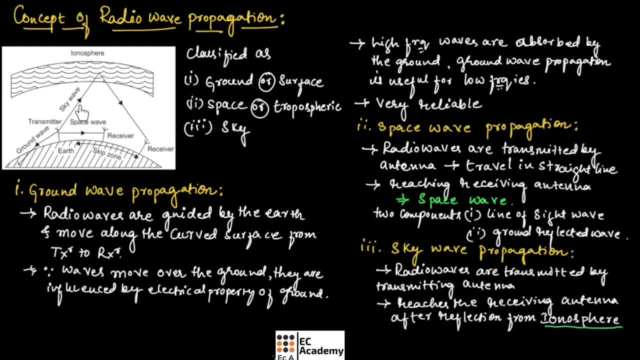 So, as you can see from this diagram, in sky wave propagation the radio waves will be transmitted by the transmitting antenna. It is reflected by the ionosphere, Then it will reach the receiving antenna. This process is known as sky wave propagation. This is about the concept of radio wave propagation. Hope you have understood the topic. Thank you.